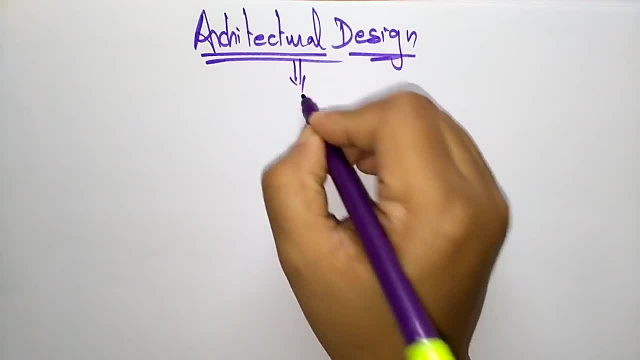 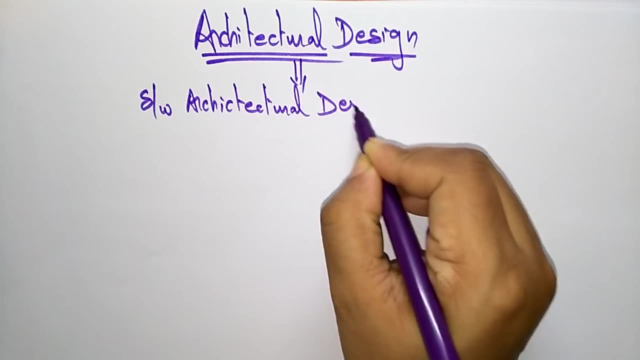 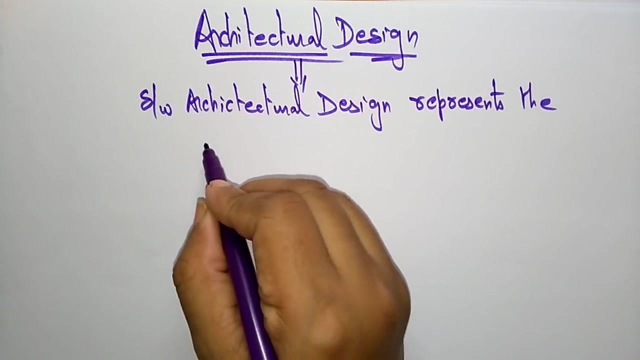 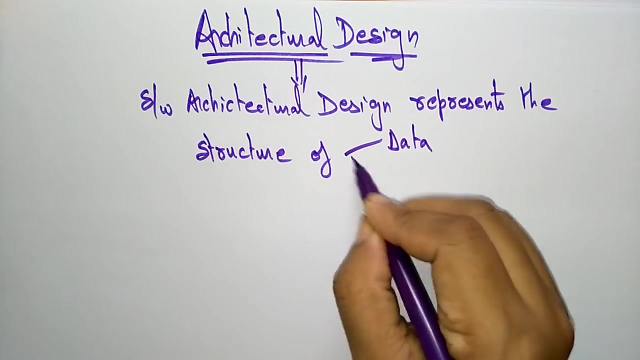 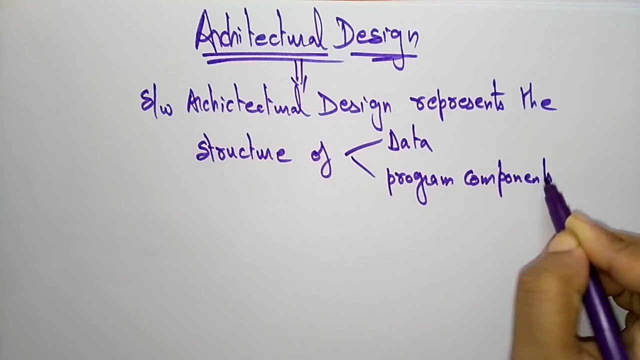 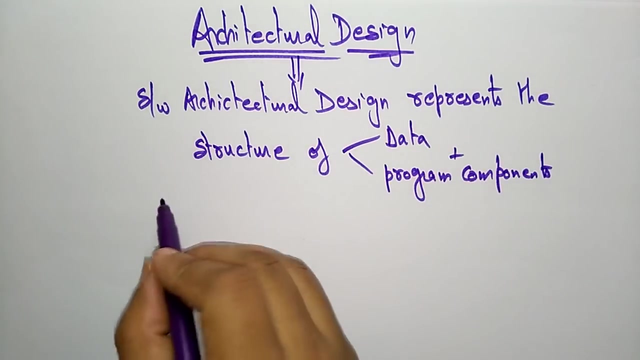 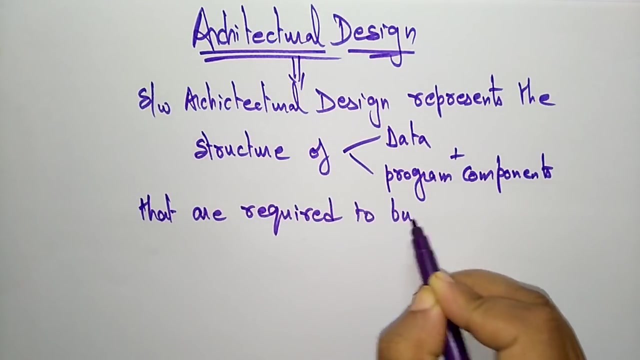 architectural design. so the software architectural design. let me write the point first. the software architectural design represents represents the structure of it, represents the structure of data and program components. so the software architectural design represents the structure of data and program components that are that are required to build a computer-based system. 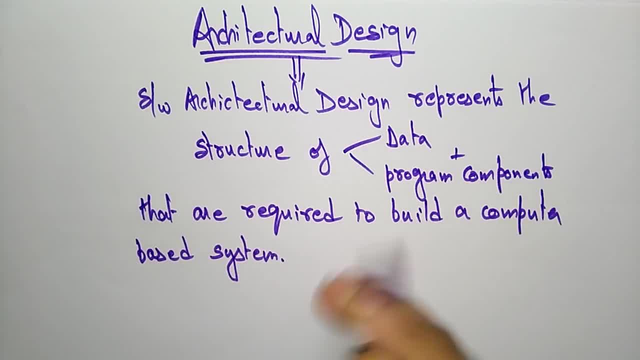 so if you want to build any computer-based system, you need the structure of data and program components that are used in the, which represents the software architectural design. so if you want to design any software architectural, first you need the structure of data and program components that are required to build a. 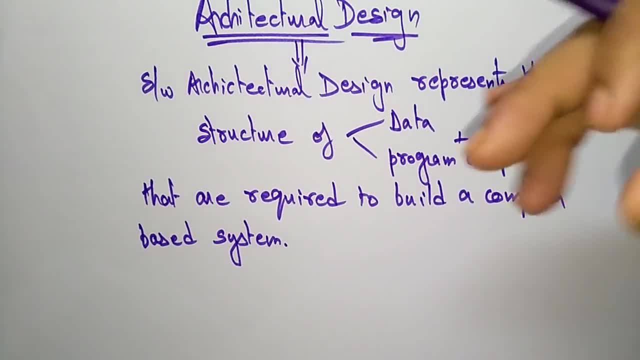 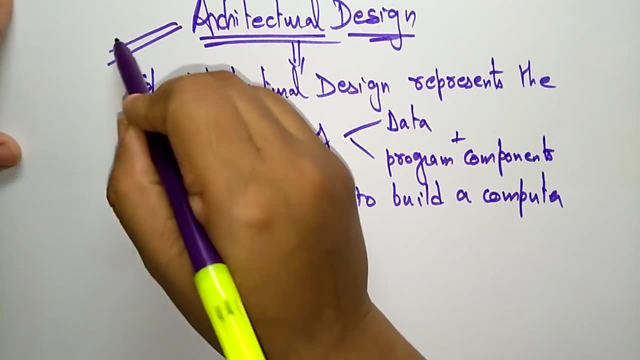 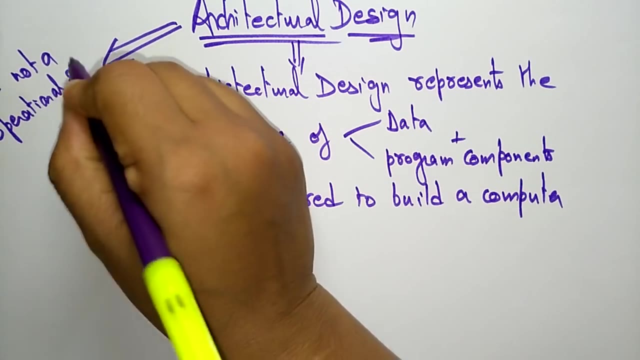 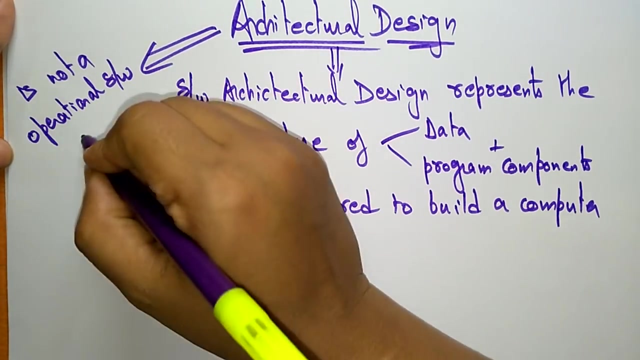 computer-based system. so actually, why we require this architecture? so first you have to know that it is not an operational software. the architectural is not a operational software, we already know that. that. but it is not consisting of any code. okay, so architectural is not a operational software. 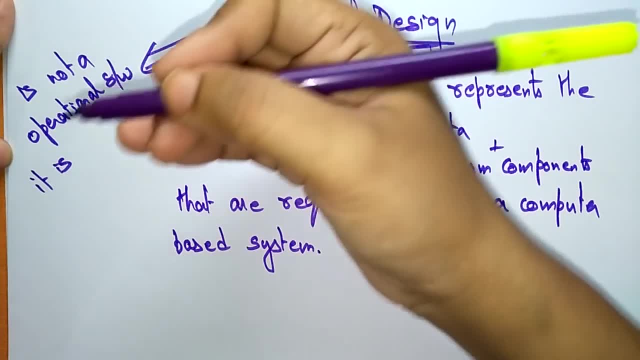 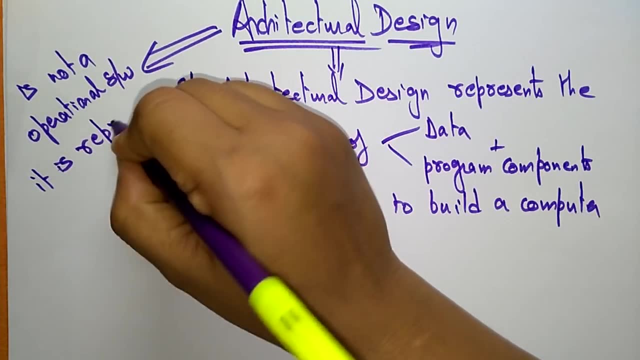 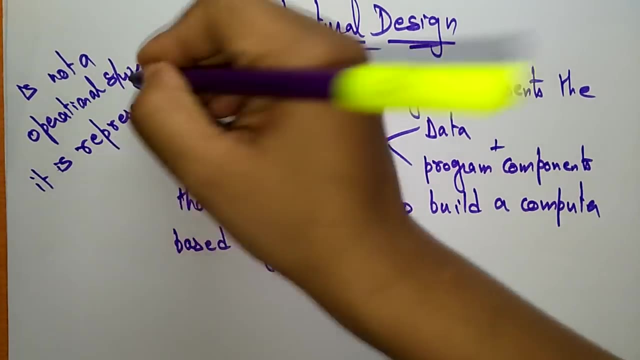 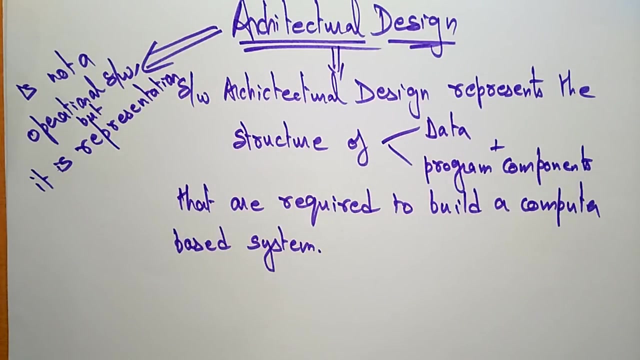 it is. it is just, it is representation that enables a software engineering. it says representation, it is representation. so it is not an operational software, but it is representation means it is a structure that enables the software engineering to analyze the effectiveness of the design, to consider architectural alternatives and to reduce the risk. 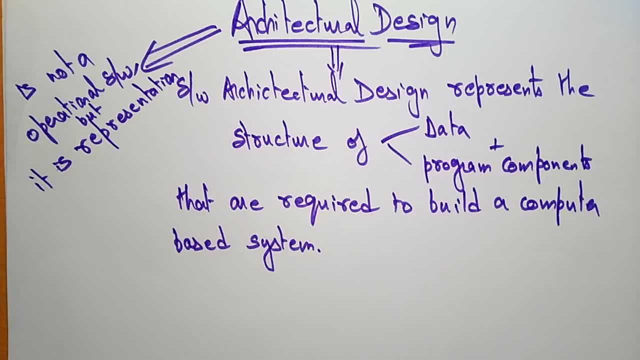 so, for all that things, the architecture design was introduced. so the first thing you have to be note that architectural design is not an operational software. it is just a representation, it is just a blueprint, it is just a structure. okay, so whatever the requirements we are taken from the customer, so that requirements have to be represented in some structure, so that 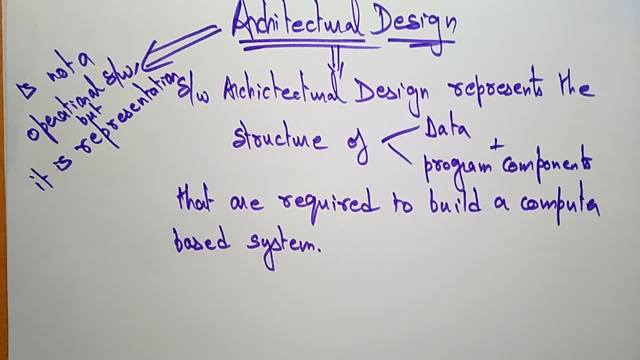 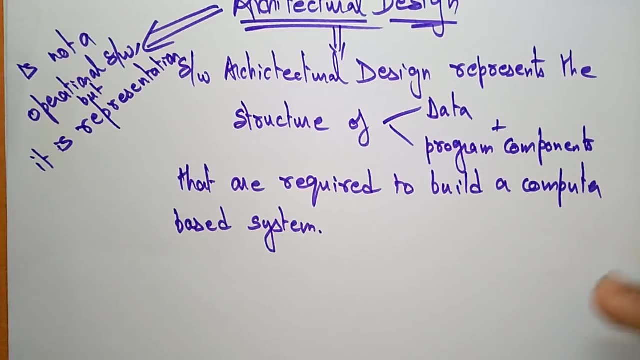 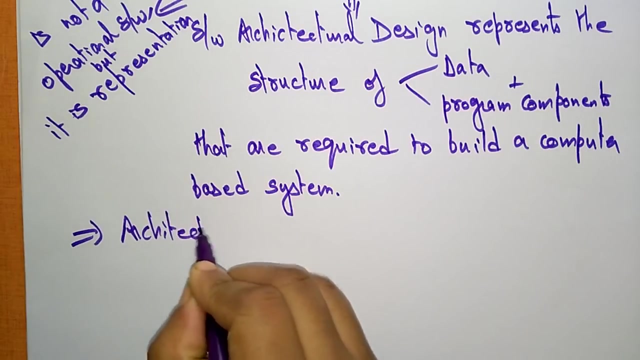 architectural design represents the structure of data and the program components that we are used to build a computer-based system. so that is just introduction of architectural design. so the architectural design representing the system in you- let me write that point- architectural design representing the system, representing the system in context. 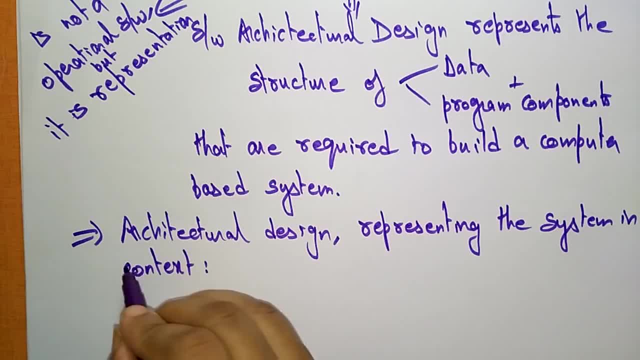 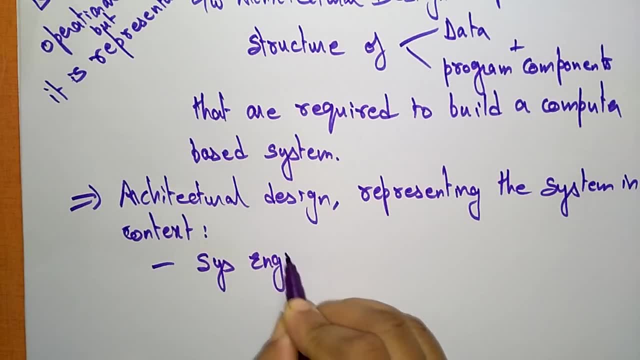 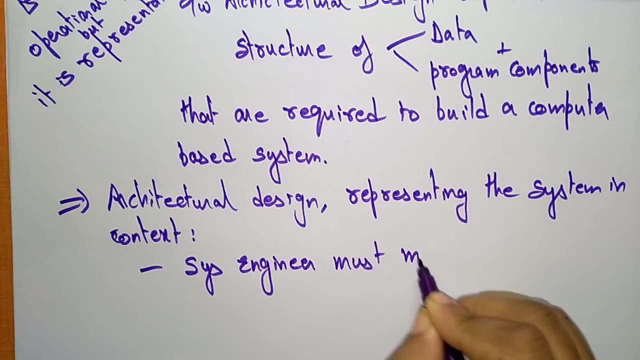 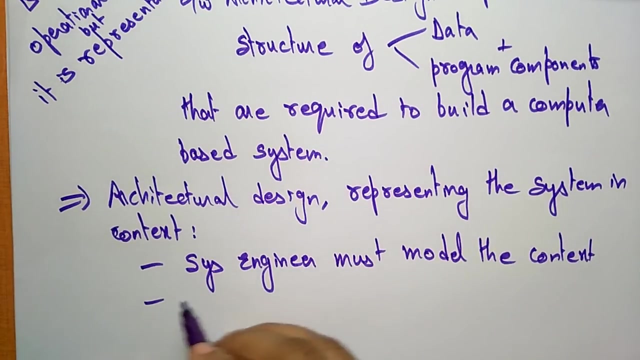 in context, that is, the system engineering must be represented in a context. the system engineer must model the context. first the system engineer, who is able to develop the system. the system engineer must model the context. so first he has to model the context, next the context diagrams that have he has to be created. so what are? 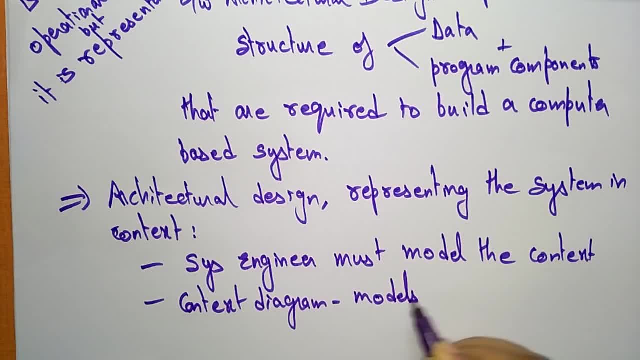 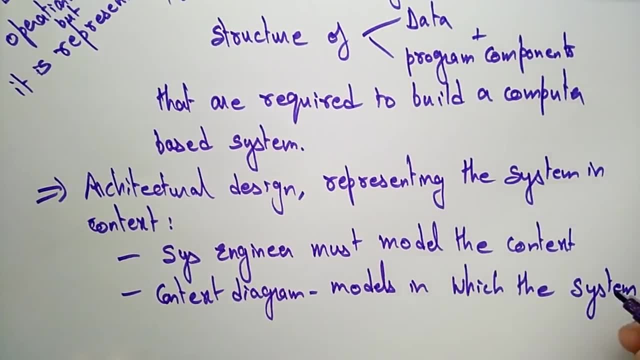 the context diagrams the models in which the systems runs on the different. the systems runs on the different. the systems runs on top of the 보� estable cucumbers. that is the philosophy of CAD in rc'sอน ned interacts the models in which the system interacts with external entities. so what? 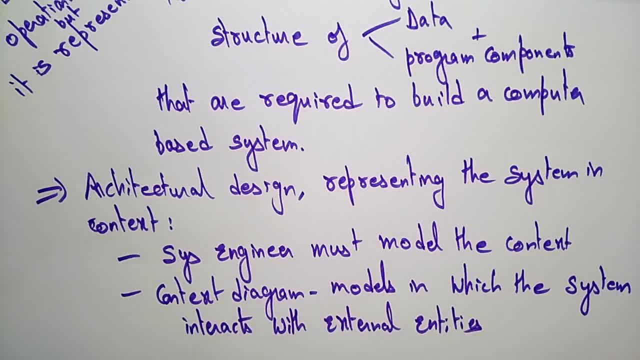 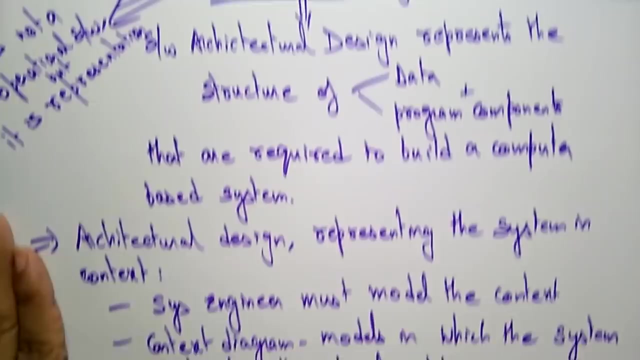 are the external entities here, the system we are going to develop a model so that, whatever the system that we are building, that system should interacts with the external entities. the external entities like uses, architectural context diagrams, input, output, user interface, processing everything. so by taking the that external entities, the system model, that is, a context diagram, will be. 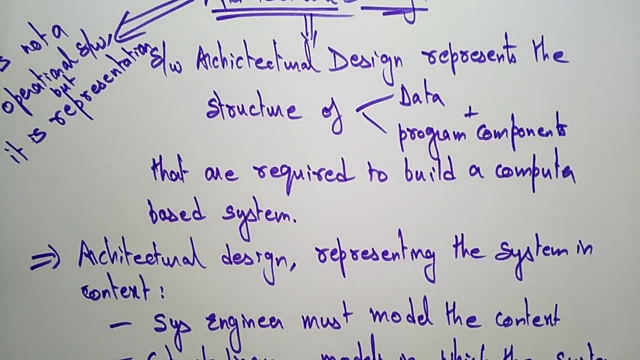 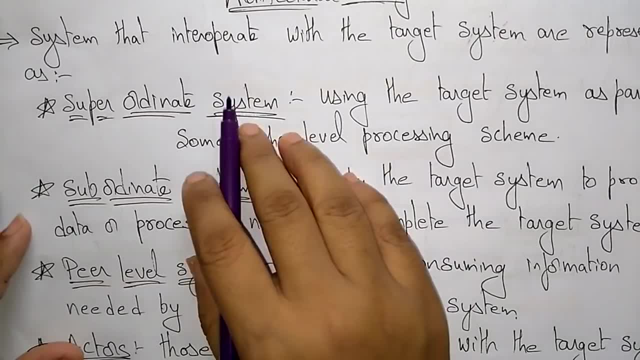 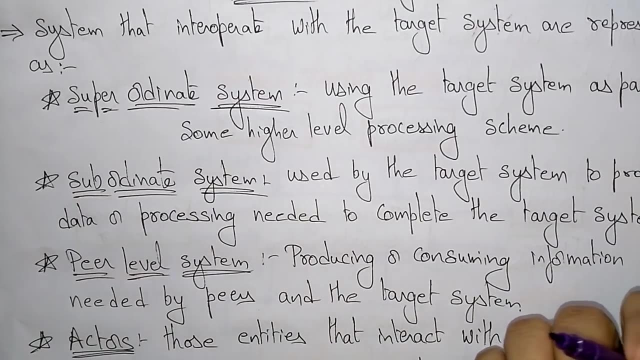 developed. so now let us see the system that interoperates. now let us see an architectural design, the system that interoperate with the target system, or represented as. so, whatever you want to implement, that it means if you take any context diagram that you want to implement. that means if you take any. 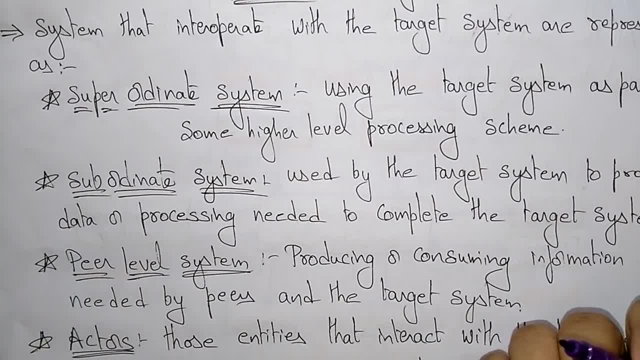 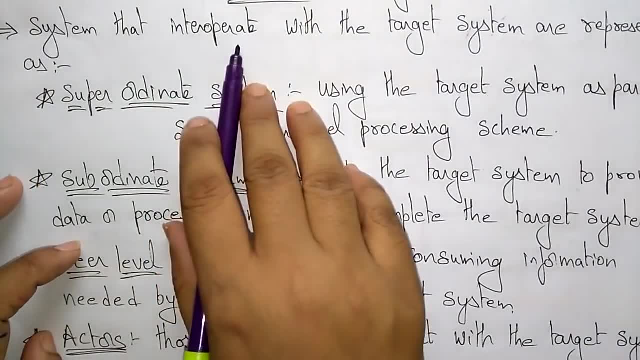 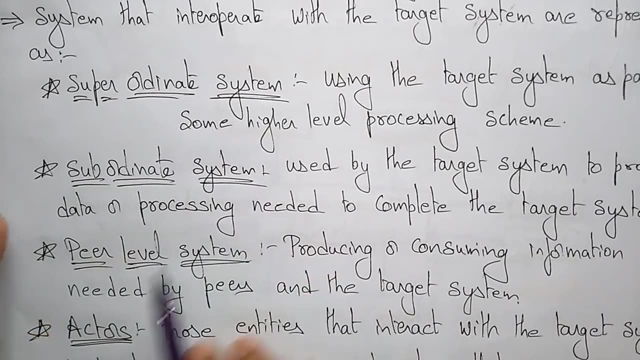 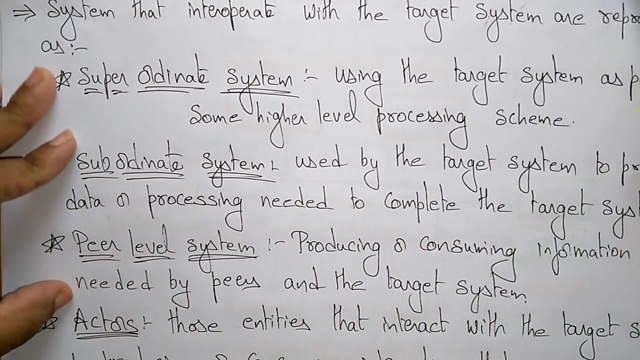 context. if you want to implement that context in by using some architectural design, you have to follow some concepts. that is, the system that interoperate with the target system are represented as superordinate system, subordinate system, peer level systems and actors. so these are the some characters or the stages that are present in any concept, in any program, so that you are going to be 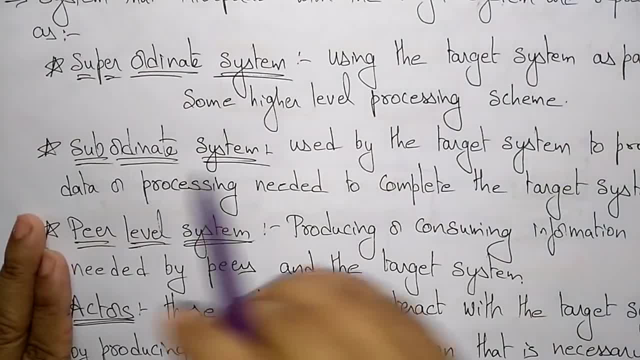 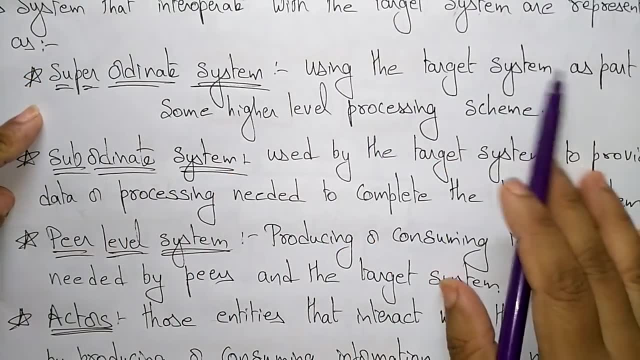 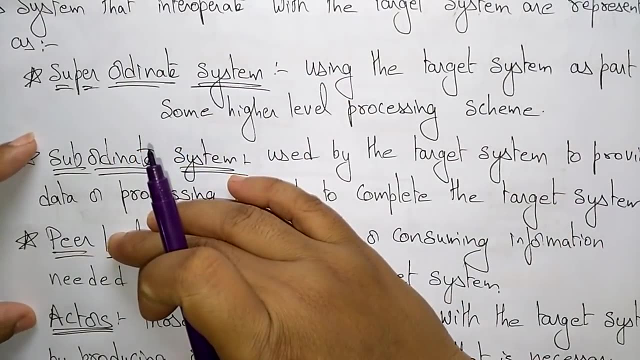 represent by using architectural design. so what is a superordinate system? the superordinate system is nothing, but it is using the target system as a part of some higher level processing scheme. so all these systems will interact with the target system. so the target system is a main system which 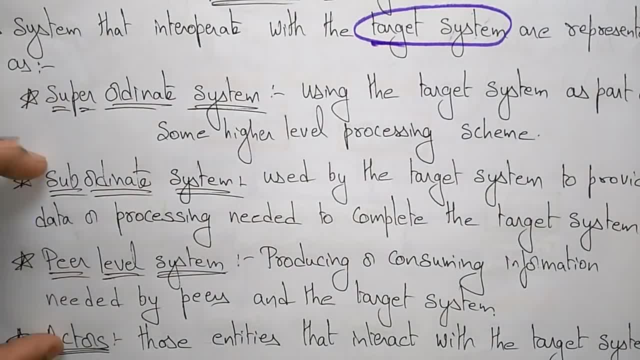 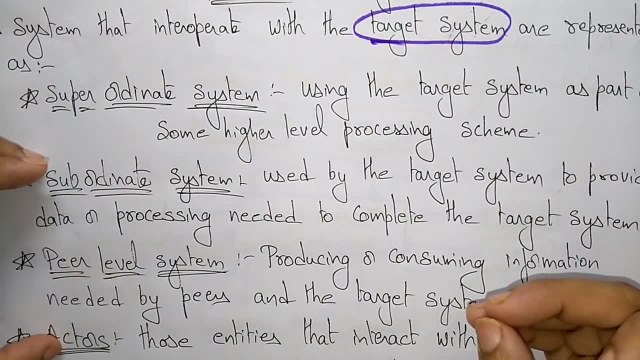 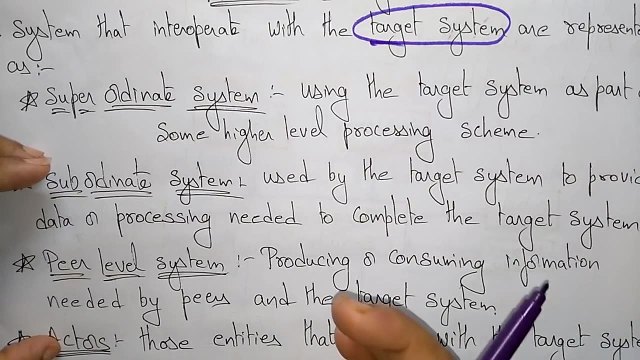 it gives the output, so that all these systems will has to interact with the target system. so, whatever the concept you have taken, whatever the requirements you have taken, whatever the product that you are going to be implemented, first you have to think about the target system, so, and next you have to. 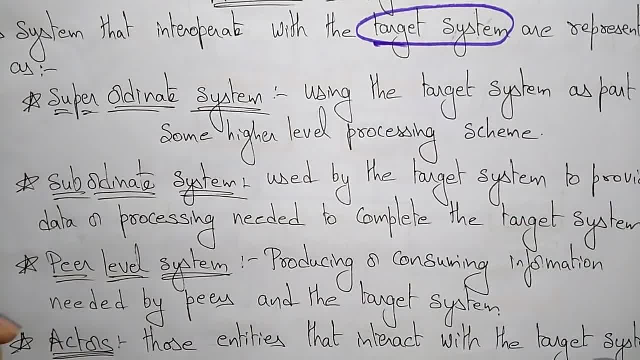 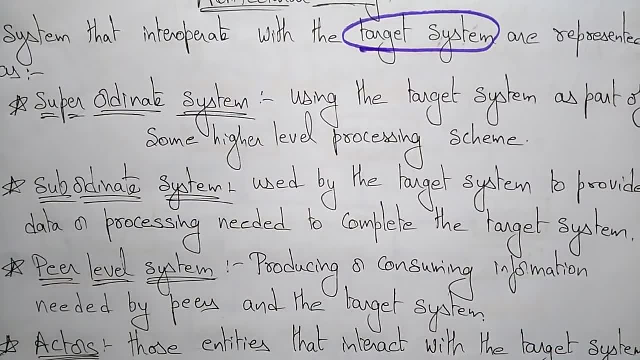 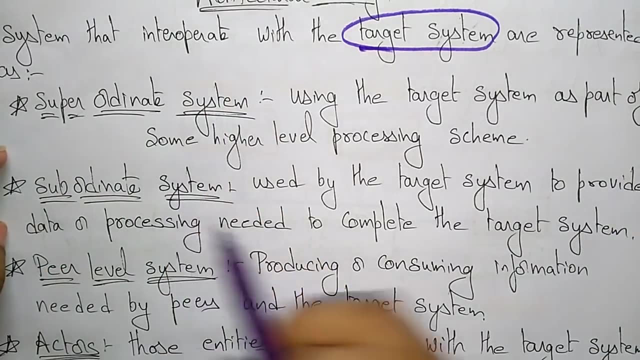 think: what are the different systems that are interacting with the target system, so that you have to be represented everything by using architectural design? so the different systems that are related to the target system. that has to be decided by using superordinate system. okay, you have taken one. 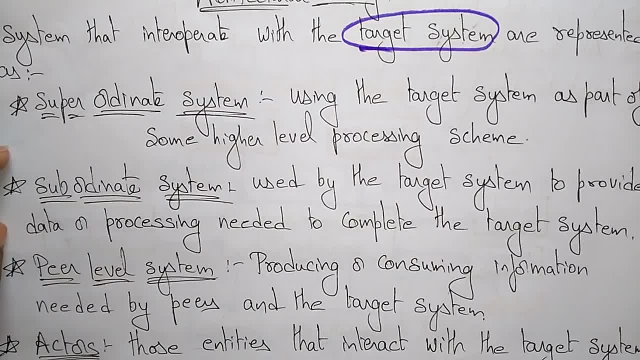 product that you are going to be implemented. suppose if you want to create in any app. so if you want to create that app, first you have to think about the target. what is the target that make it as one system. then in that app you have to be decided who is the superordinate system and who is the 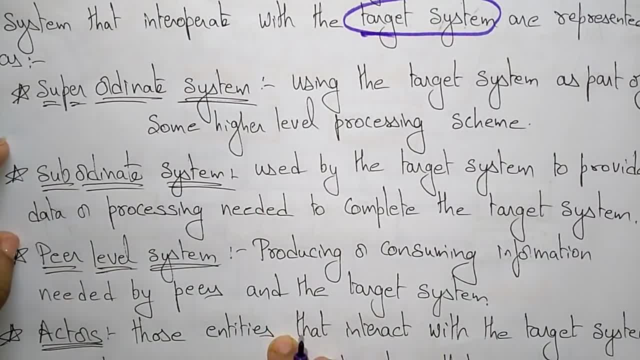 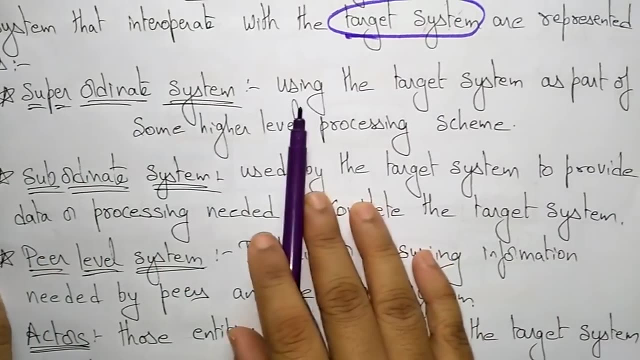 subordinate system and who is the pr level system and who is the actors here? who is? it's not a man, it is a system. okay, it is a modules. just think about it's a modules or it is a components. the superordinate system is nothing, but it is using the target system as a part. 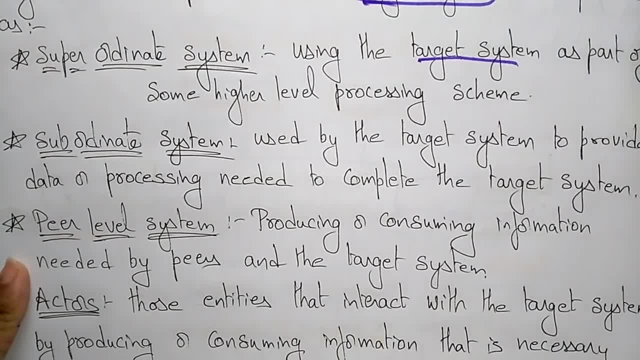 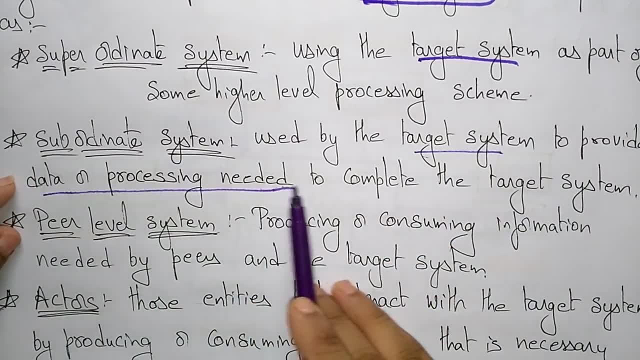 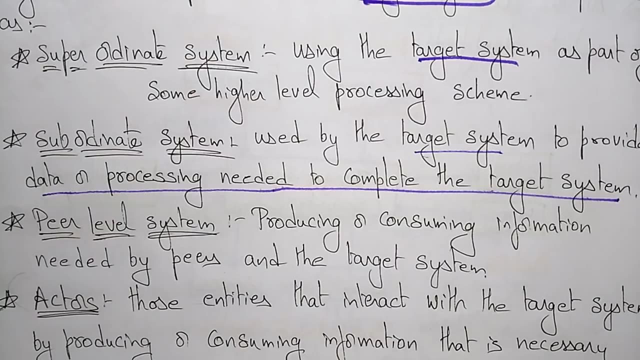 of some higher level processing scheme and next to the subordinate system. the subordinate system is used by the target system to provide data or processing needed to complete the target system. okay, if the target system want to achieve some output. so, with the help of this subordinate system, the target 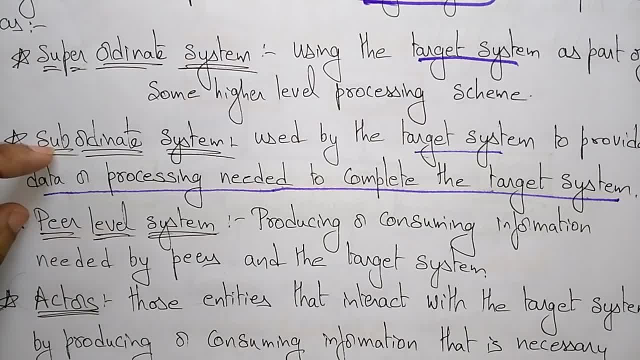 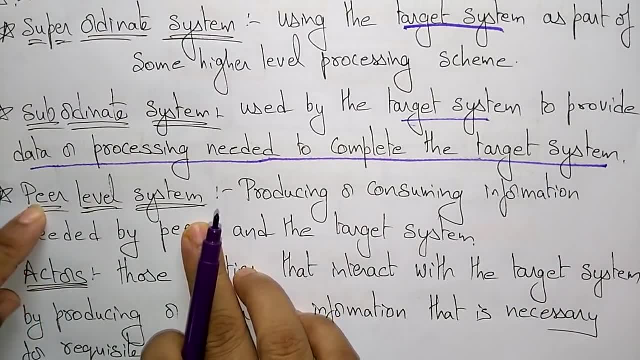 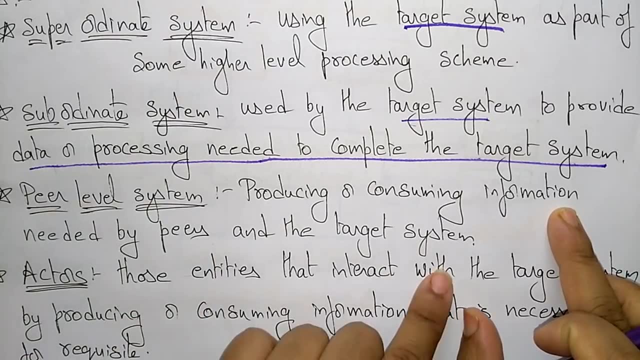 system. the target system can complete its need with the help of data or processing, which is provided by the subordinate system. next is a peer level system. so what is this peer level system will do at the peer level system? producing or consuming the information needed by peers and the target system. so the 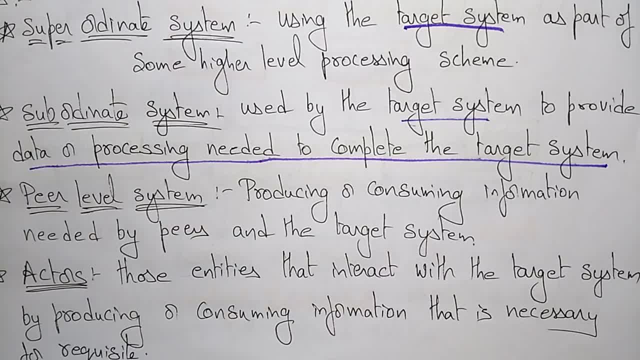 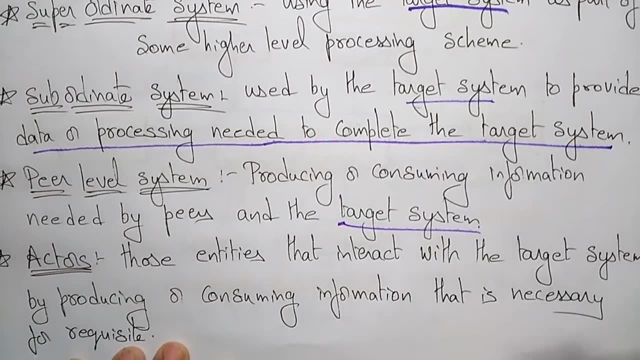 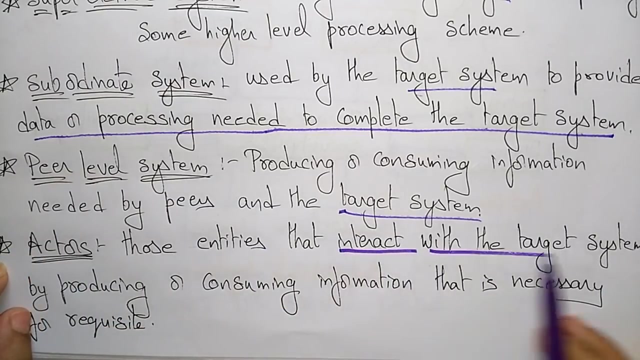 peers will need some information means they wants to the peers or nothing. but the users- okay. so those people, those peers, wants to produce or to consume the information by them and at the same way, and the target system next is the actors- will present the actors or those entities that interact with the target system. so this you have to be remember: actors. 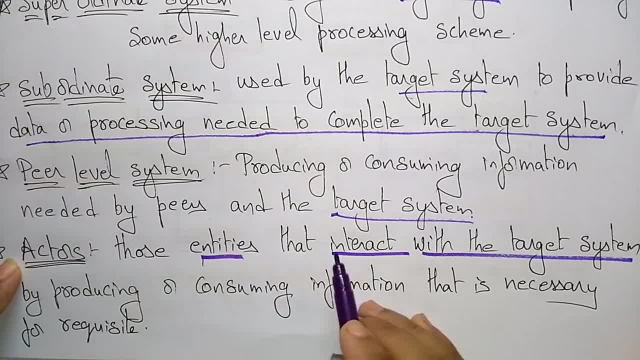 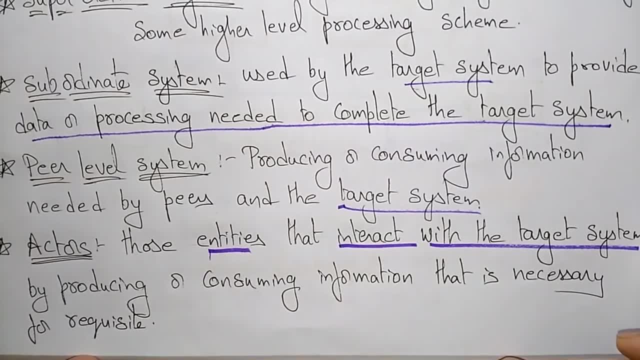 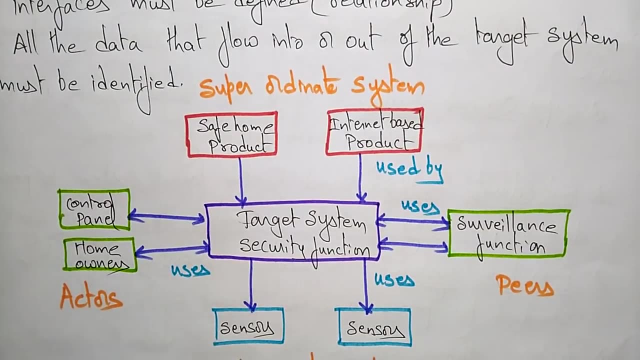 are nothing but the entities that interact with the target system by producing or consuming information, that the, the, that is necessary for requisite. and here in this architectural design, after, if you find, after finding out the subordinates, superordinates and actors, and the peers, next is the interfaces. 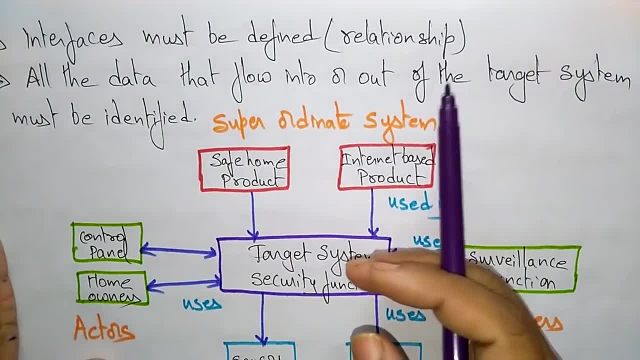 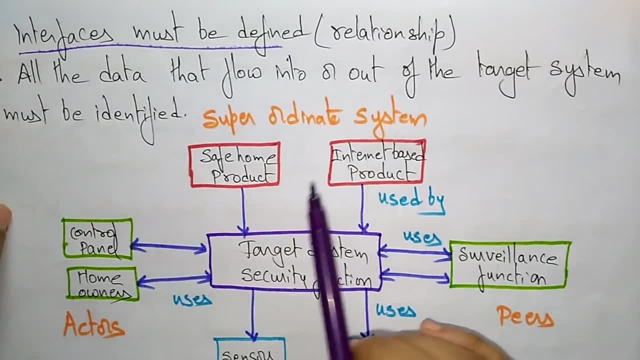 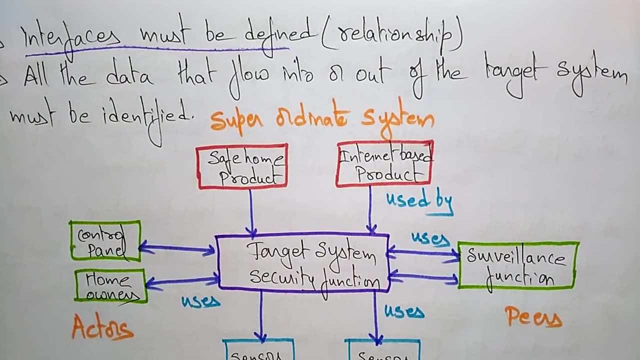 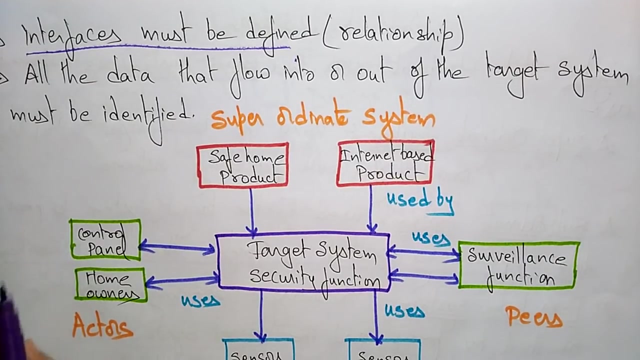 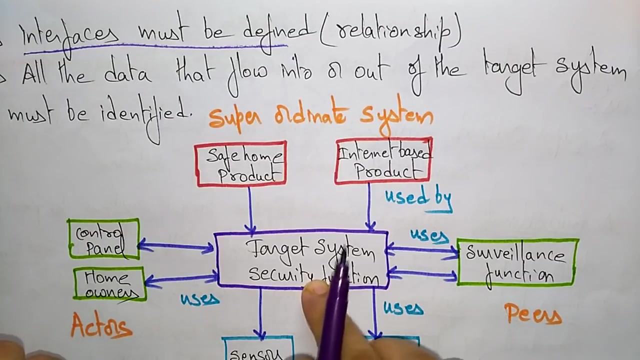 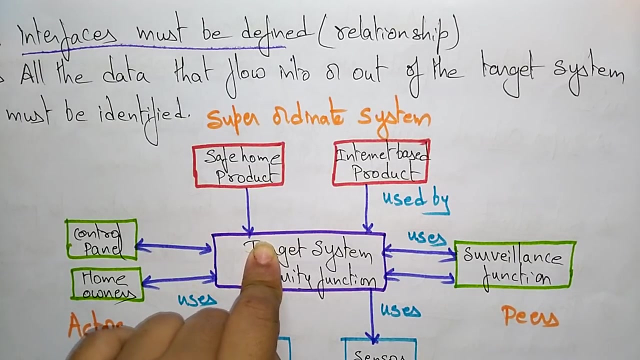 must be defined. so there should be a communication, there should be a relationship between those systems. so next you have to find out. the interfaces must be defined, that is, the relationships. after that, all the data that flow into or out of the target system must be identified. okay, next you have to think about from where to where the data is going means from. you have to identify the input flow and as well as the output flow. so all the data that flow into or out of the target system must be identified. so this is a target system. so from here the data will: from where we are getting the data and from where we are sending the data, to which system we are sending the data that has to be identified. so this is a target system. so from here the data will: from where we are getting the data and from where we are sending the data, to which system we are sending the data. that has to be identified. so this is a target system. so from here the data will: from where we are getting the data and from where we are sending the data, to which system we are sending the data that has to be identified. so this is a target system. so from here the data will: from where we are getting the data and from where we are sending the data, to which system we are sending the data. that has to be identified. so this is a target system. so from here the data. 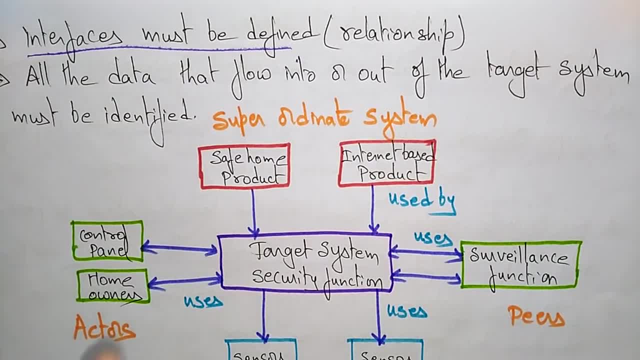 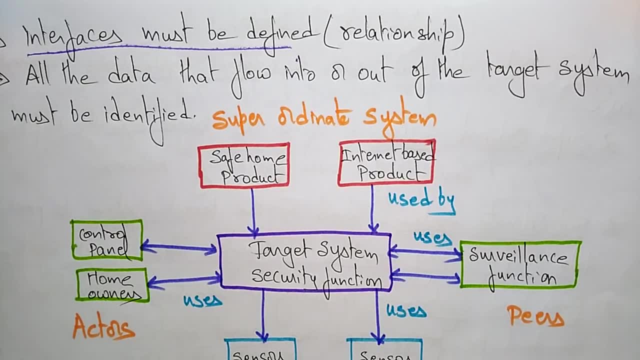 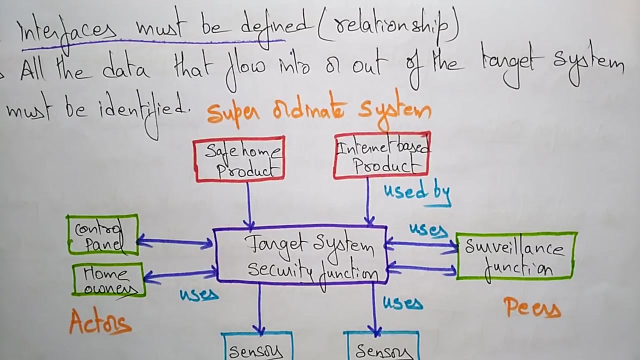 is a process of architectural design. so if you want to develop the by using architectural design, if you want to construct anything, if you want to structure the representation, you need to fast. first you have to identify the superordinates and the subordinates and the actors and the peers that are present in your system and the target system that is present. so after that you have to interface, you have to establish a relationship between those systems. 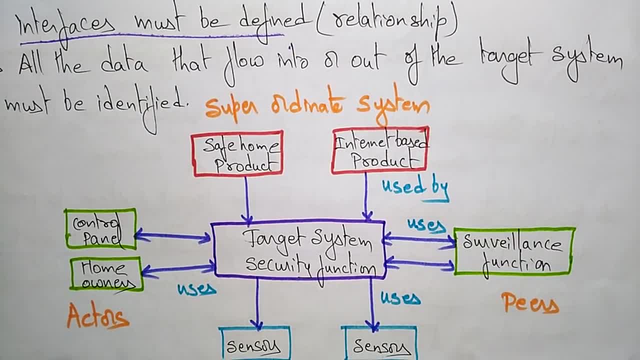 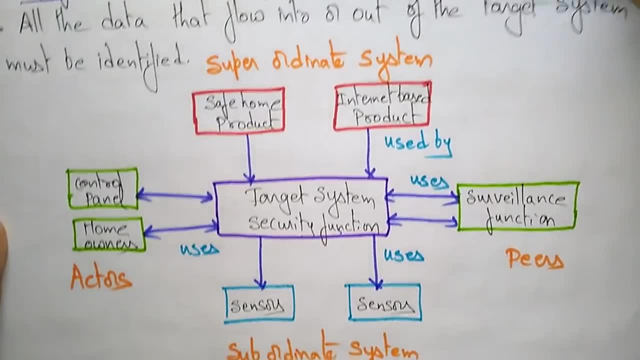 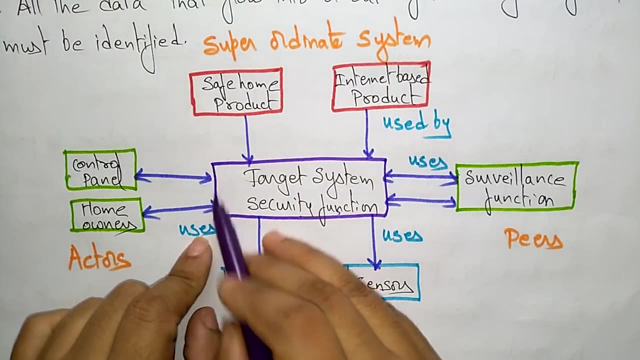 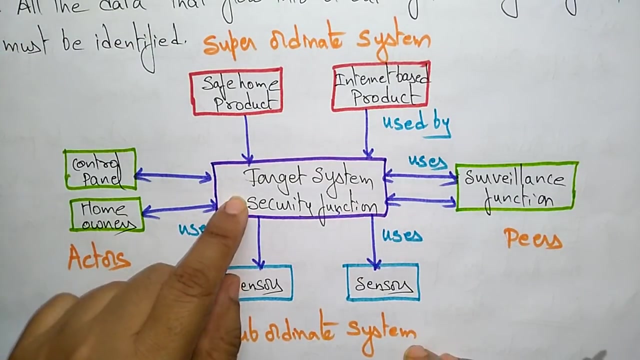 after that you have to identify the data flow into or out of the target system. okay, so here you can see. this is the target system security function. here I am taking a security function that is a CC cameras as an example. the target system is a security function, is there? so to operate anything, everything should has to, has to interact with the target system. first let us think about the superordinate system. so in this, 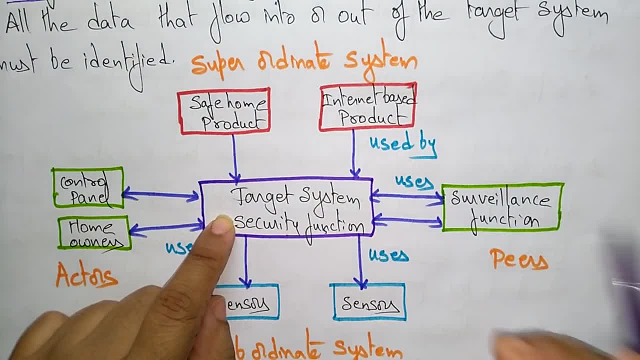 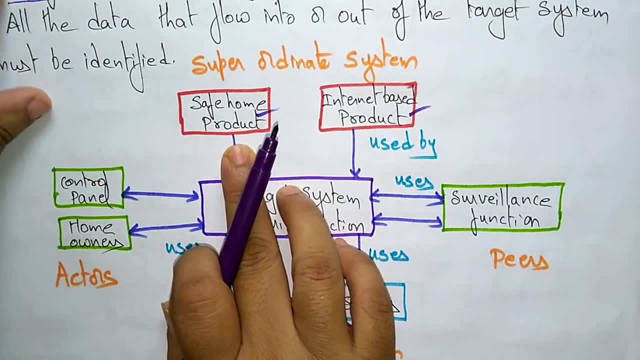 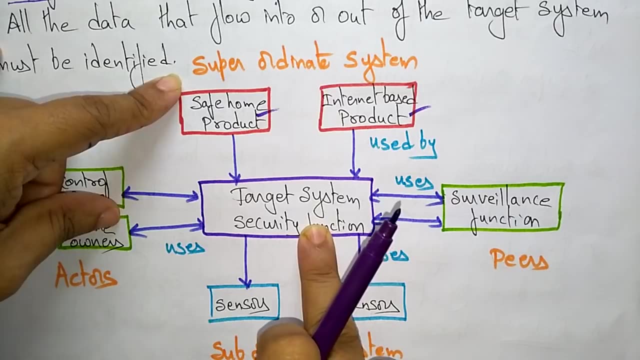 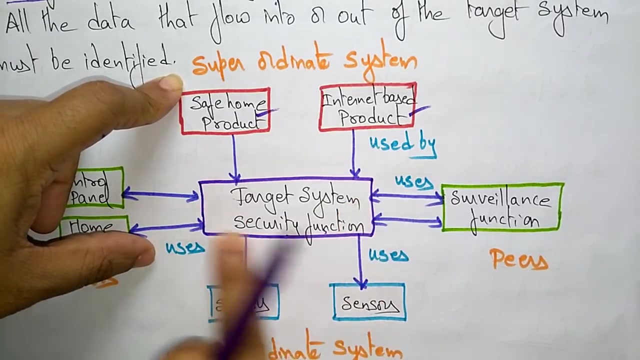 security function. so who are the superordinates? the superordinates are nothing but the safe home product and internet based product. so these two are the comes under the superordinate system. so what I said: the superordinates are nothing, but they are using the target system as a part of some higher level processing scheme. so this safe home product and internet, internet based product, or using this target as a higher level processing scheme. and next is 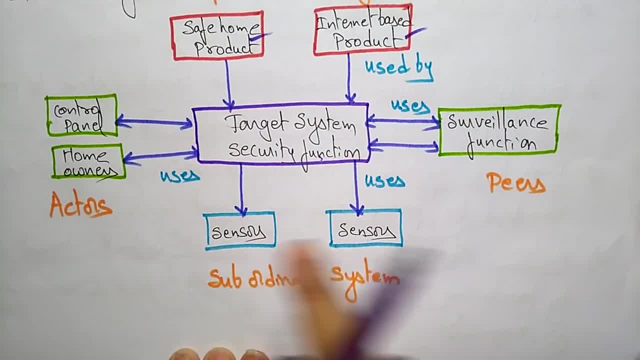 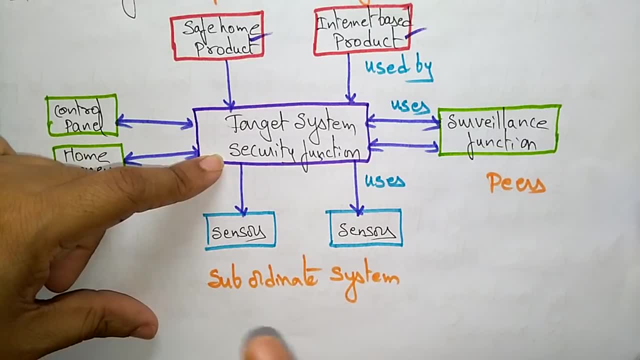 subordinates. so who are the subordinates here? the sensors are acting as a subordinates for the target system security function. so what do you mean by subordinate system? the subordinate system used by the target system to provide data or processing needed to complete the target system. so to complete the target system function, this sensor will be used. so that is a subordinate system. now, coming to the peers: who are the peers here? the peers are not.